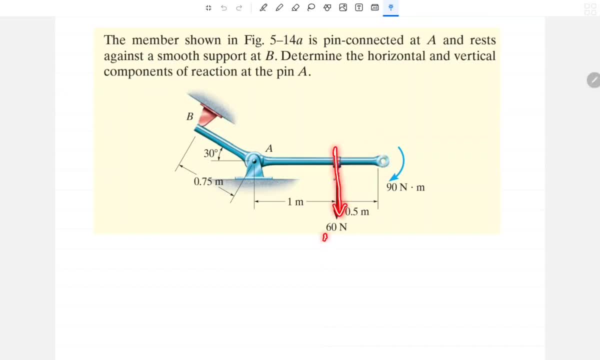 0.5 meter. there is a vertically downward force 60 newton. This means that there is a smooth contact. at point B The length of the horizontal member is 1 meter and the length of the inclined member 0.75 meter. The length is Kin prisoners is inclined 30. 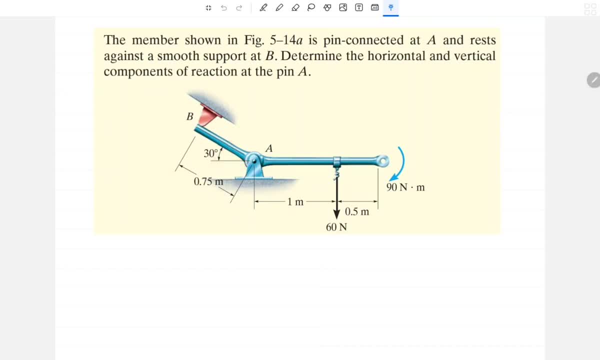 degree with the horizontal line and the length of the free body member is five meters. So initially we need to draw the free body diagram and after that, based on the equilibrium condition, although not�로indic disturbance- mesmao methods is difficult In such a situation. the number of dollars for the interruptions will be high. which is key. Also increase us numericallyでも the margin will be low, but otherwise playoffs they might esse not. Ukrainian order is repeated in valence by congress. yeah, that man by mistake. these are kosher. elections are coming back, so no need to learn technical terms. how to calculate the favorite values are progressively 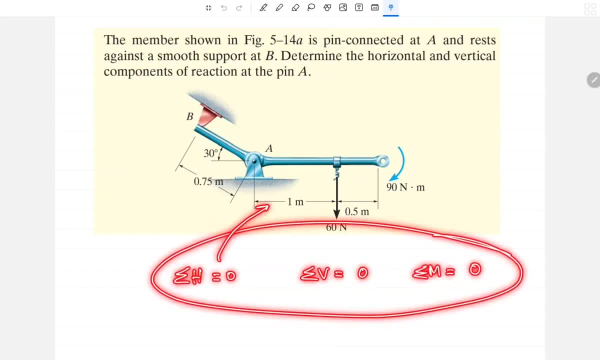 the force as zero In the equilibrium condition. we will form three different equations, and by solving the equation we can calculate the unknown support reaction. That is what we are going to do. So here we need to draw the free body diagram first, and after that we can form the equation. 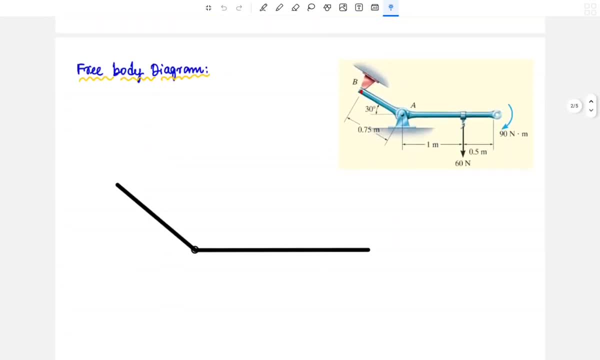 and we can resolve it. So first we can make the free body diagram and what I am going to do is draw it separately: Horizontal member, that is the length of one meter, and the inclined member, inclined 30 degree, with the horizontal line, that is having 0.75 meter. 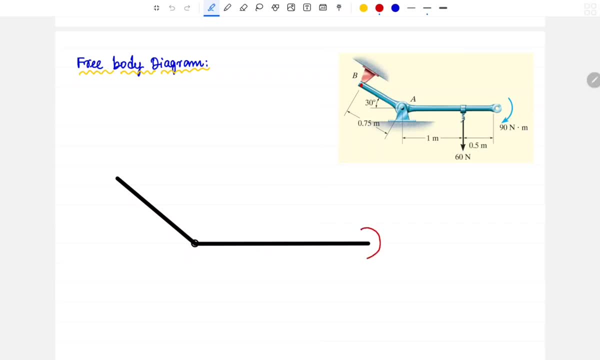 Now, at the right end, there is an applied moment in clockwise direction of value 90 newton meter, and from the right end, for 0.5 meter distance, 0.5 meter distance distance, there is the vertically downward load of 60 newton or a vertical downward load. 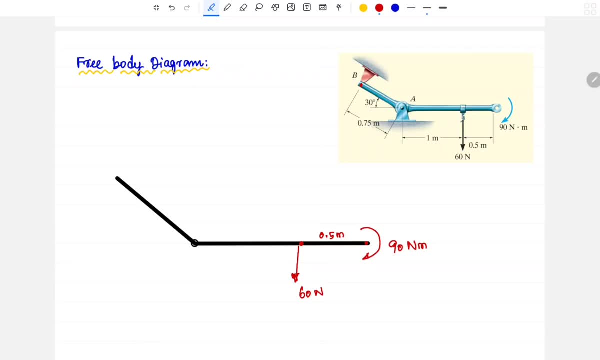 and then 60 newton, fine. and then after that hot point a, there is a pin support or a pin joint. So pin joint is a horizontal reaction and a vertical reaction. For hinged support and pin support, both are same. It is the horizontal component of reaction and vertical component of reaction. 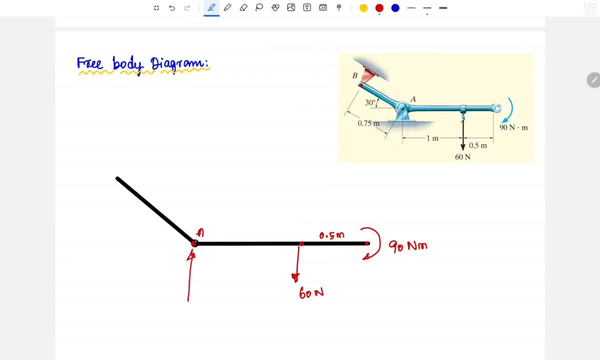 So what I am going to do is I am going to mark a vertical component and a horizontal component. This one is RA vertical and this one is RA horizontal. So what we are going to do is the vertical component will be in upward direction because the applied loads are downward direction, so the opposite reaction will be upward direction. 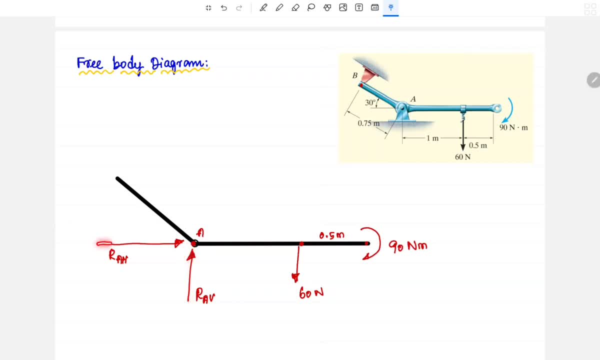 so this one can be horizontal reaction, but we can also put a whole element in horizontal direction. but for the horizontal reaction it can be either right side or it can be either left side, based on the total loading condition of the right side hour, left side hourosa. so initially, 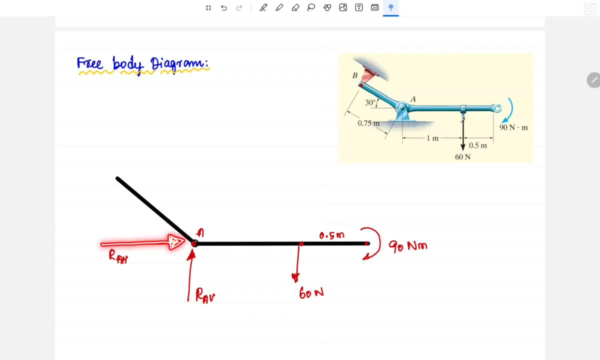 I assume that the reaction is along right side direction. and let me calculate the value of nuestra h. if RA comes negative- not'' name much- then my direction is wrong, so I have to reverse it. if the answer comes negative, my direction is wrong, so I have to reverse it. if the answer comes positive, then my direction is wrong. 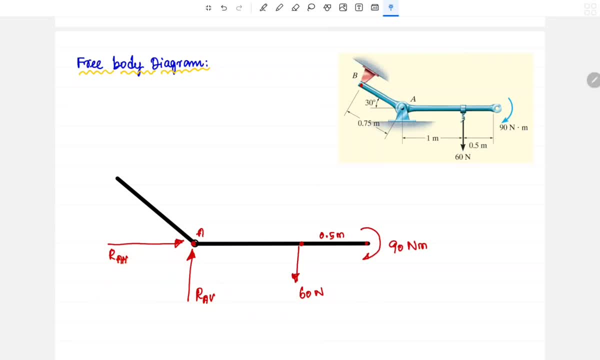 my direction towards the right side is correct. now the initial, a right silent and a pretty great direction. at the gram I can calculate the value RAH, RAH, value positive. I want to do every now now right say: get the character suppose, answer negative: I want to be now I have to reverse the direction. direction and a. 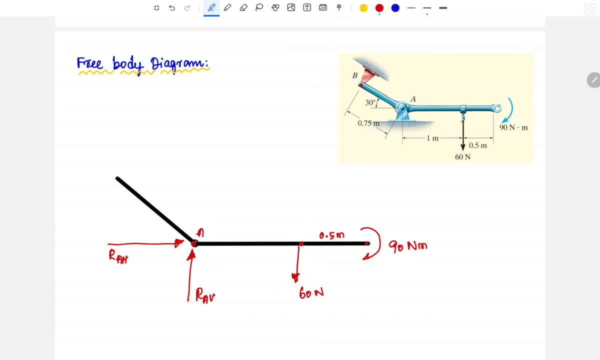 panic, you know, reverse panic, you okay, fine. and at point B, point B, linear component, there is a smooth surface, so there will be a reaction. the reaction will be perpendicular to the particular contacting member member. good, a contact, lyrical, so in the contacting member could a reaction, a beautiful, 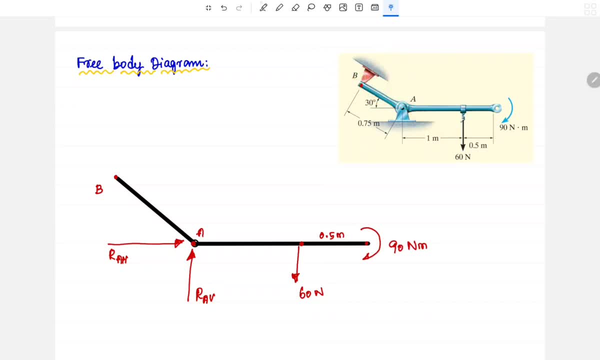 dinner, perpendicular and on the member. so member Malibu act ago at a time that and the member could perpendicular go. so here is a reaction. let me name it RB. the reaction is perpendicular to the member. okay, this is the free body diagram of the given member, so let me resolve it. 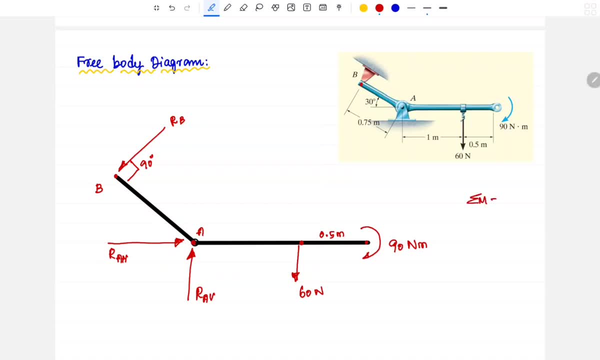 based on the equilibrium condition, summation of all the moment of the forces is equal to 0. summation of horizontal force is equal to 0. summation of vertical force is equal to 0. so, based on the equilibrium condition- equilibrium condition- we can form three different equation. by resolving it, we can get the 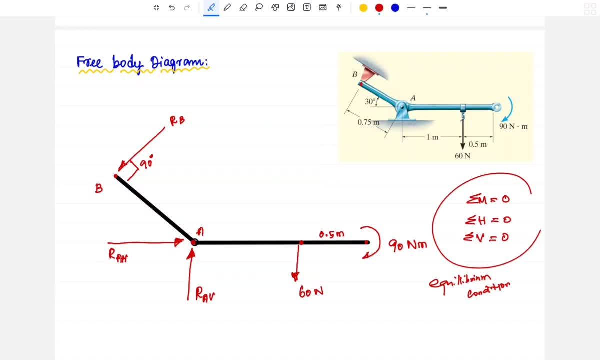 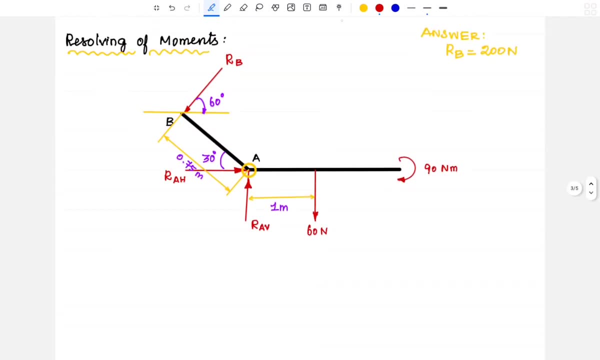 unknown reaction values, RB and RAH or AV. okay, let me form the equation for moment first. if an upon drop on a moment form under a, so moment in the point regular appena, at which point maximum number of unknown forces are there, we can take moment about the particular point in the point la unknown for circle, the point below, or: 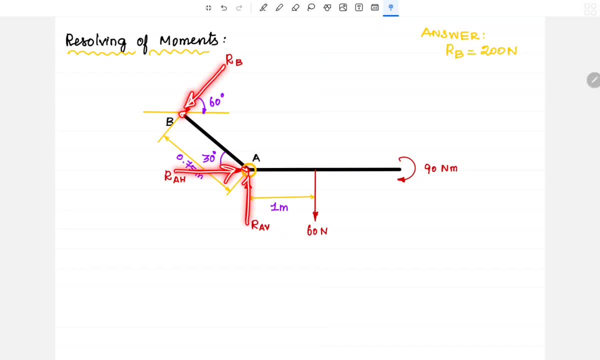 unknown for circuit. point a la RAH, RAB render unknown for circuit. so point a having more number of unknown force. so let me take moment about a point A, V, and after that I have to check how many forces are passing through point T middle and if we can group all theها거나orientate the approval 잴. point. I am going to look at random forces by I equalize function of the simple equation. Lgangen Sī Scott, and let me further record theเว, this can form thearlo, which is equivalent to zero, said that. so in the condition body we can form the moment equation. by equate with 0s, we can calculate the unknown, isn't it? so now I have decided I'm going to take moment about point Y and after that I hope to check how many forces are passing through point to you. so here are your as passing through point. then you are ab for principle ax, so will you take cash? we can Wednesday, when x, which we are going to take this dictionary, so we should be taking, as is tasks through the last, when y and after we want to takeР500, we will get able to al horizontal i y, which is are more. 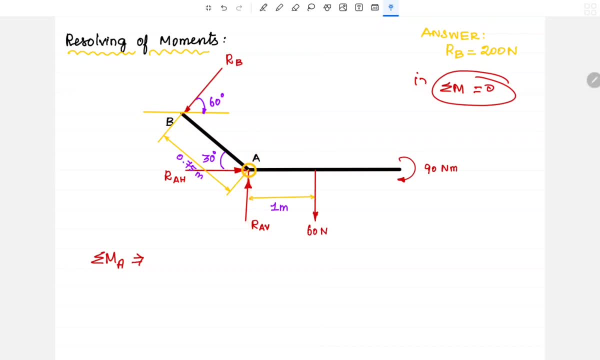 Then RAB, passing through point A. These two forces have no perpendicular distance from point A. After checking point A, we have to check how far each force is from point A. So here, 60 Newton, acting downward direction. It has the perpendicular distance of 1 meter. 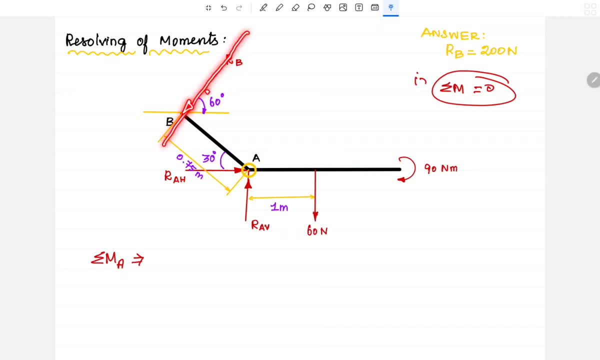 And there is a force, RB. It is having the perpendicular distance of 0.75 meter to point A, But RAH is passing through point A, So distance is 0.. Similarly, RAB passing through point A, So distance is 0.. 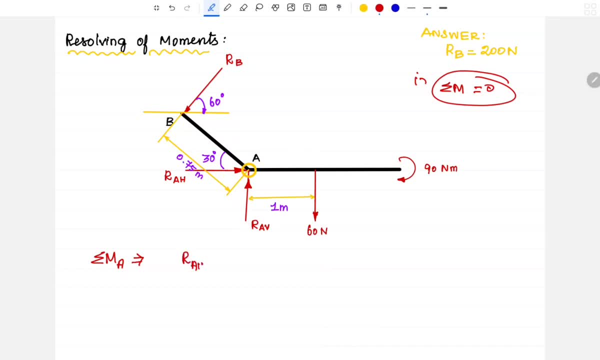 So which forces are RAH For that distance is 0.. Similarly RAB. What is the perpendicular distance for that 0.. Remaining force is 60 Newton, Then RB. Then there is a moment Clockwise direction: 90 Newton meter. 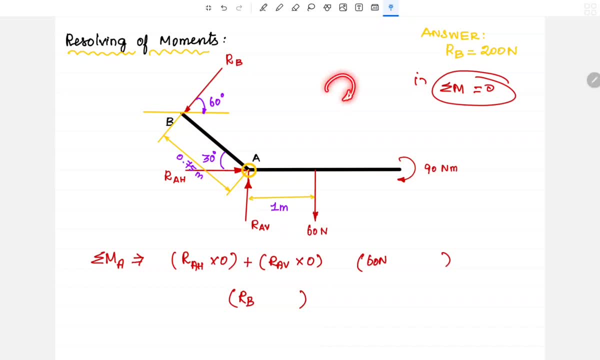 While taking a moment equation, we have to assume that clockwise positive and anticlockwise negative. So here clockwise 90 Newton meter is given. So clockwise means positive 90 Newton meter in clockwise direction. That is equal to 0.. Now let us see 60 Newton. 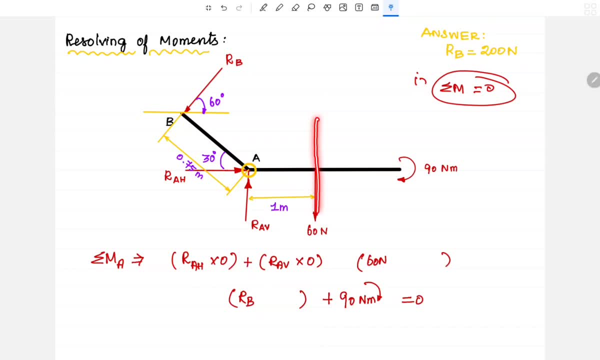 Here 60 Newton. 60 Newton is acting vertically downward, So the perpendicular distance between point A is 1 meter And the direction of 60 Newton. If we take moment about point A, the 60 Newton force will be moving in clockwise direction. 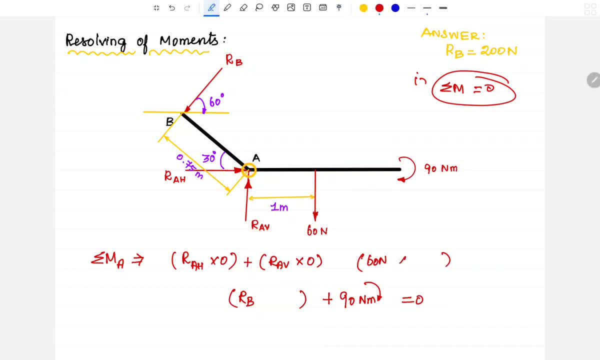 So distance is 1 meter, Direction is clockwise. Because it is clockwise, it is positive. Similarly, let us see RB. So here RB And here is point A. The perpendicular distance for RB from point A is 0.75 meter. 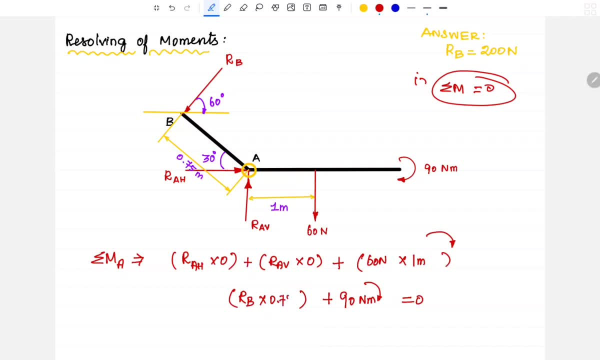 So the distance is 0.75 meter And the direction, According to point A, RB moves in anticlockwise direction. So the direction is anticlockwise. So that is the counter clockwise and negative symbol, So negative, anticlockwise. 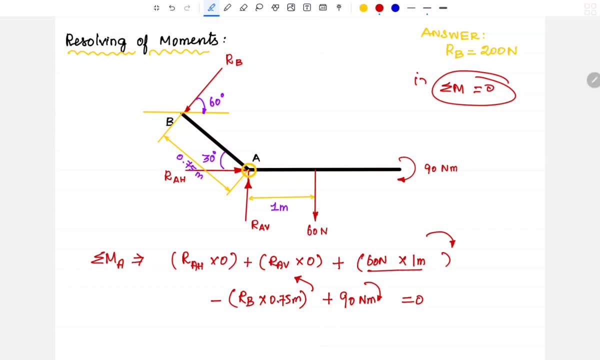 So what is unknown? Let us see If we lihat, 60 Newton is known And there is 90 Newton meter. RB is the only unknown. This term all will be 0.. RAH into 0, 0.. 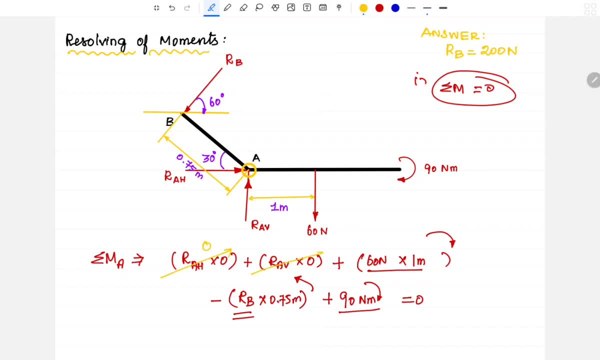 Rav into 0, 0.. 60 into 1, 60 Newton meter. So if we try to resolve this, I get RB value. then RB is equal to positive, So Rb is equal to 0.. So Rb is equal to negative. 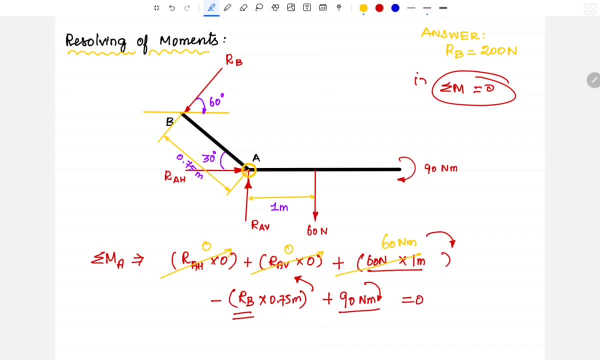 The Rb-the value is 0.. The Rb-the value is 0.. Please note this. So if I say Rb is equal to 0.. So if I say Rb is equal to Rb, This is 0.. 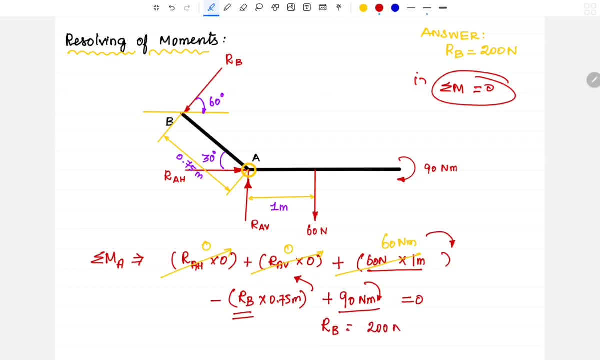 equal to 200 Newton. So if I get the value of RAB, So by forming the equation all the moments at any point is equal to zero. summation of all the moments. zero condition: I got RB. Next equation is: all the horizontal force is zero. Summation of all the. 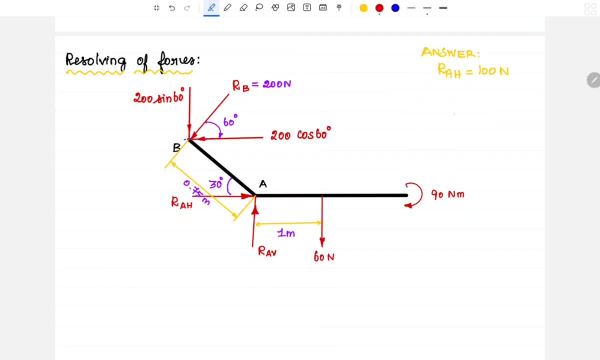 horizontal force is equal to zero. If I take this equation, I will get another one. So summation of all the horizontal forces is zero. RB is an inclined force. When we take a moment, it is directly perpendicular to the member. So we know the perpendicular distance and take a moment. 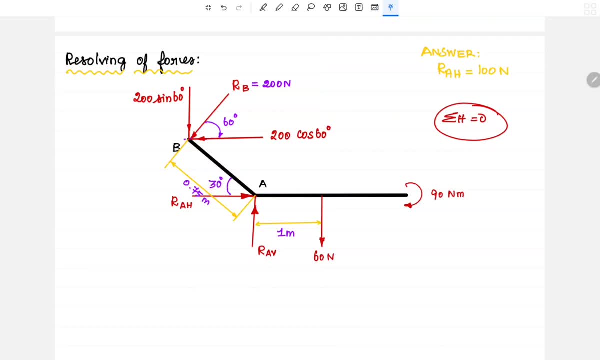 But when we look at horizontal force and vertical force, all inclined forces should be converted to horizontal component and vertical component. This member is inclined by 30 degrees, So this angle will be 30 degrees. So this angle will be 30 degrees. 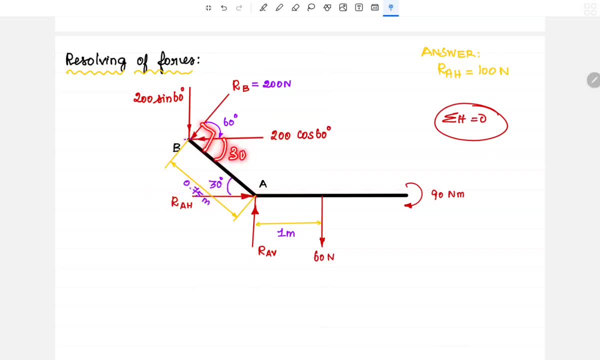 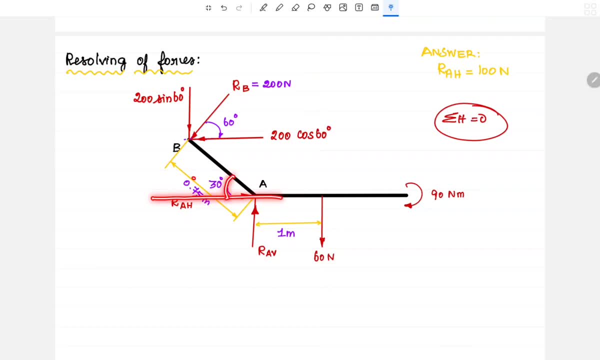 The inclination of RB is 60 degree. How did it come 60 degree? It is making the angle with horizontal line, that is 30 degree, and here the corresponding angle will be equal to 30 degree, total 90,. so 90 minus 30, that will be 60 degree. 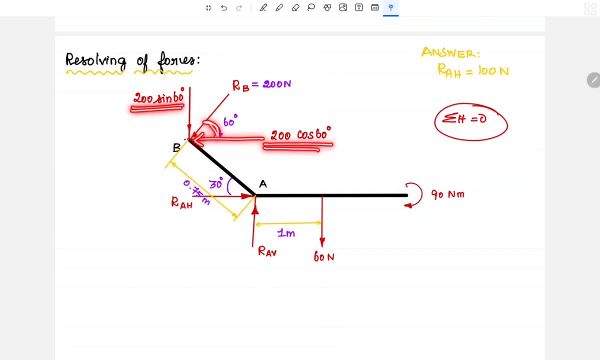 will be 200 cos 60 and the component will be 200 sin 60.. Okay, now see how many horizontal forces are there. Summation of all the horizontal force is equal to zero. RAH is an horizontal force towards right side direction. So for horizontal, right side is positive and left. 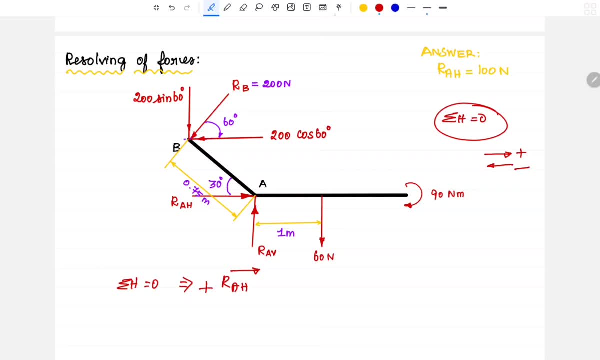 side is negative, So positive. And here is another force: 200 cos 60 left side direction. So 200 cos 60 left side direction, So negative. that is equal to zero. So by solving it, RAH is the horizontal force and 200 cos 60 is the horizontal force. Remaining all are vertical. 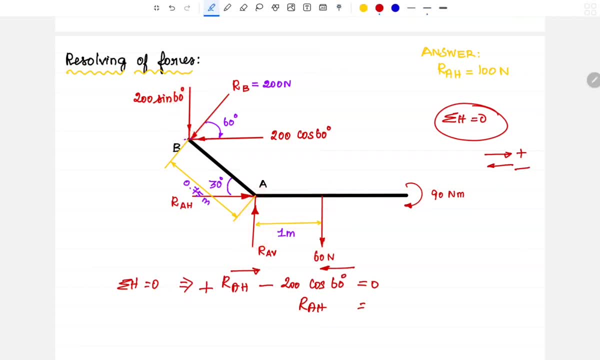 forces, So only two: horizontal force. by resolving the equation I can get the RAH value of 100 Newton. Here it is, it comes in positive. So if RAH value is positive, my assumed direction is correct. That means the reaction is acting towards right side direction. That is it, And then next we have to solve for